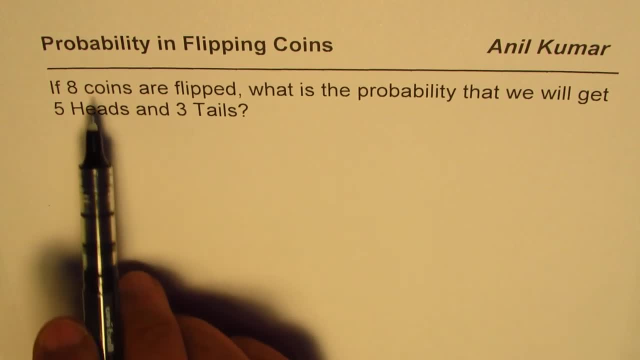 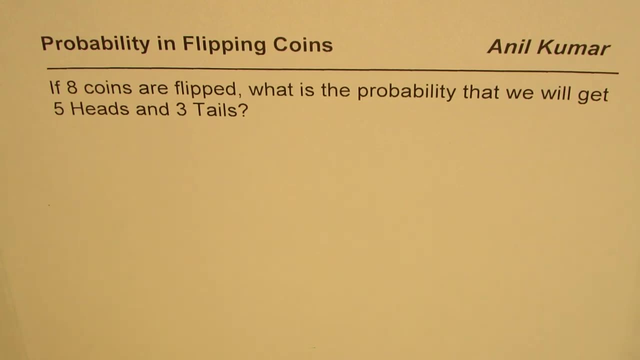 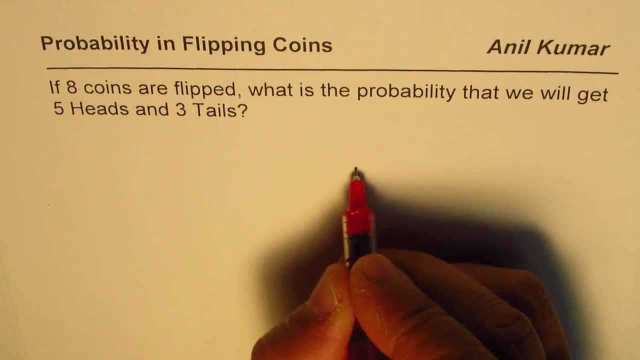 equations of coins using a tree diagram. Now, when there are too many flips, then the tree diagram becomes extremely complicated, right? So we prefer to use counting principles. So let's look into this. We are saying eight coins are flipped, So that means there are eight positions: One, two 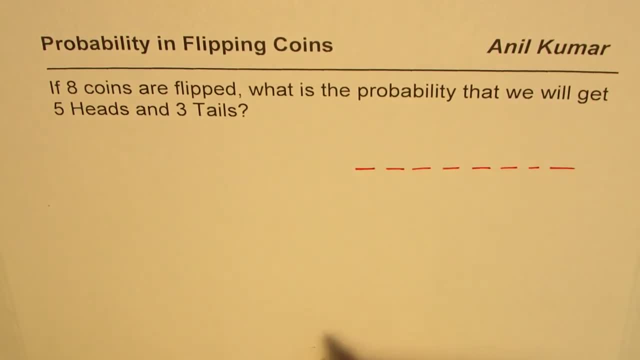 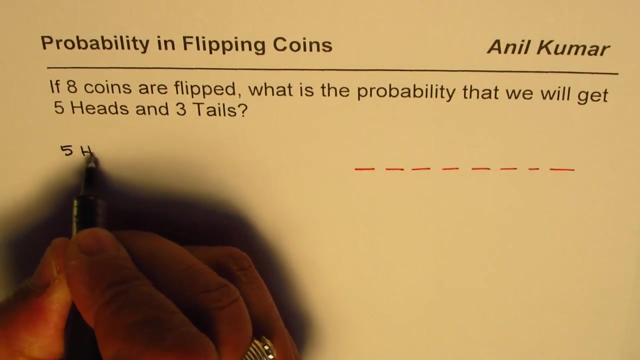 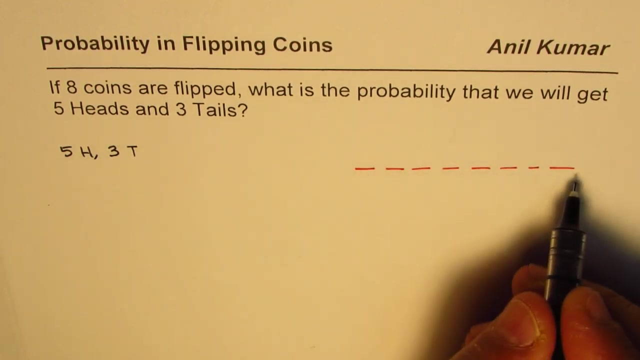 three, four, five, six, seven, eight. Now it says what is the probability that we will get five heads and three tails. Now, when we say five heads and three tails, we are saying five heads and three tails, So that is combinations eight. Now, in this case, since eight coins are flipped, total number of options which: 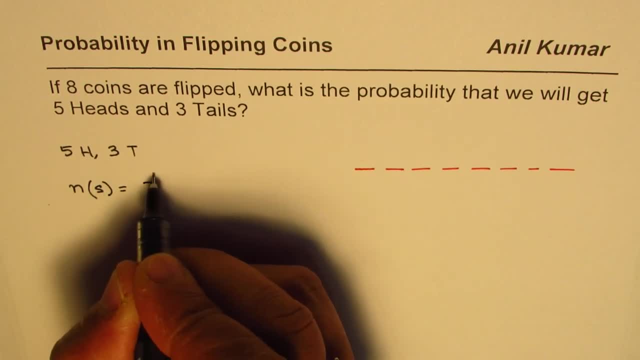 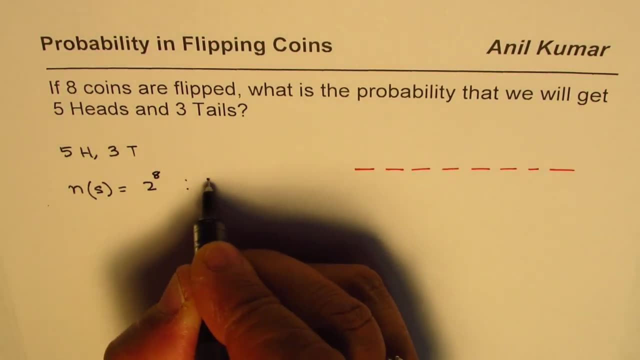 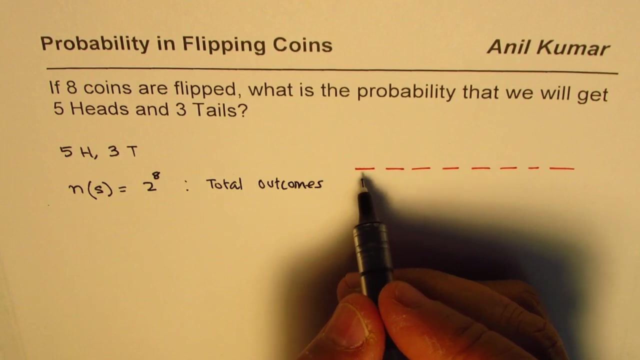 we have, that is, the sample space, is two to the power of eight, right. So those are total number of options or the outcomes, So these are total outcomes. So every time when you flip it could be a head or a tail. So writing the from the counting: 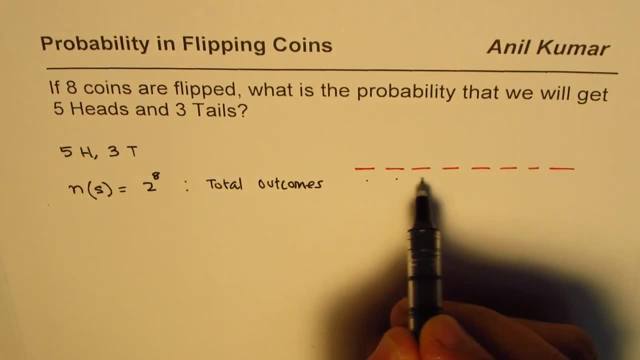 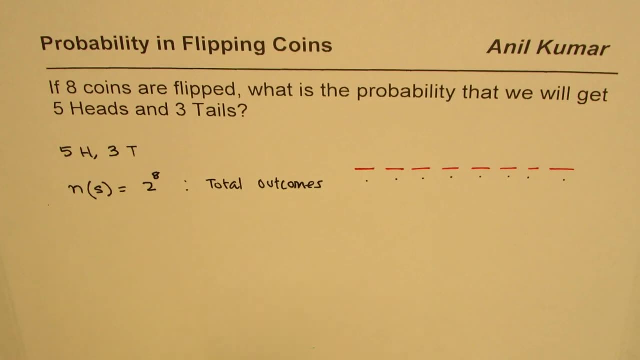 principles. they get multiplied So two to the power of one, two, three, four, five, six, seven, eight. So that gives you total number of outcomes. Now, when we are saying five heads and three tails, in that case order is not infinitive. So we are saying five heads and three tails. 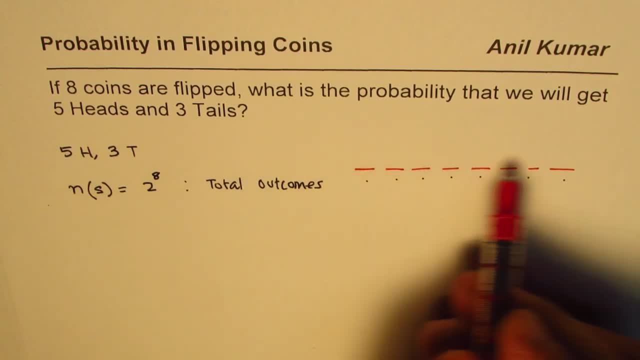 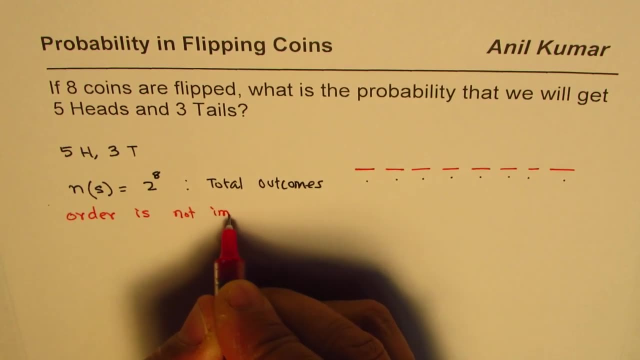 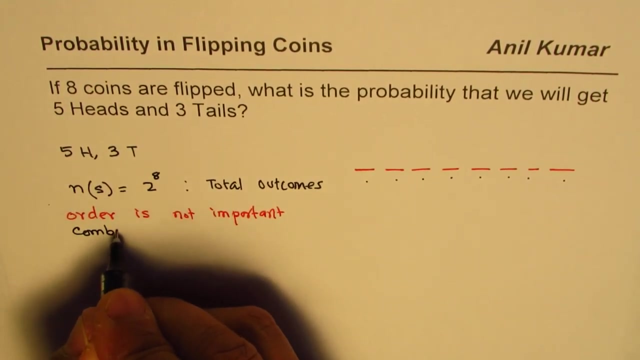 important, right? So what we consider here is: these five heads could be in any position, right? So order is not important. That means we are looking for combinations, right So we are looking for combinations, And what combination we need? We need five heads, So. 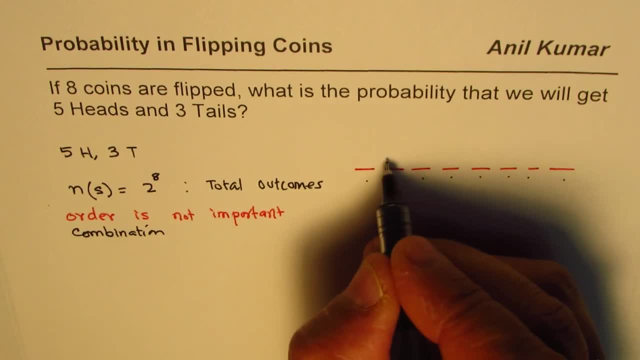 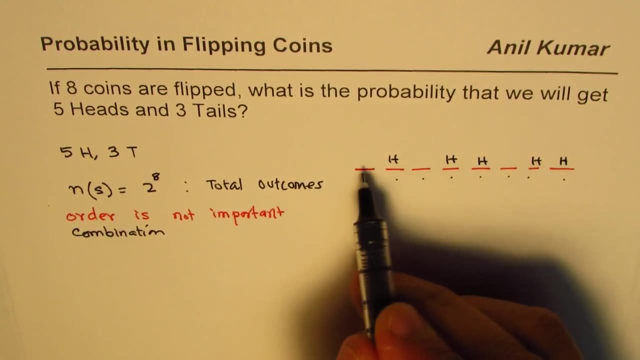 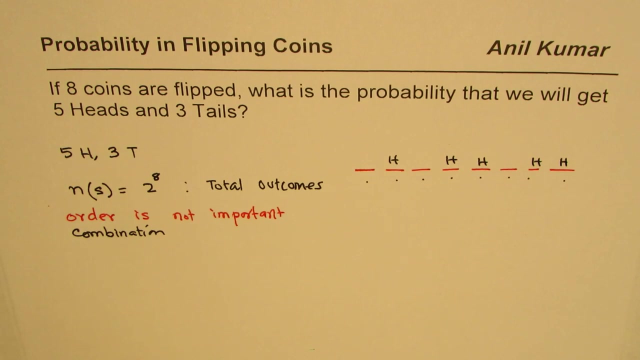 if there are five heads, we could put them in any position. Let's say one head here, one, two, three, four and five. Now it doesn't really matter where these heads are. The other blank spaces will automatically be tails, if not heads. So we are considering five heads.